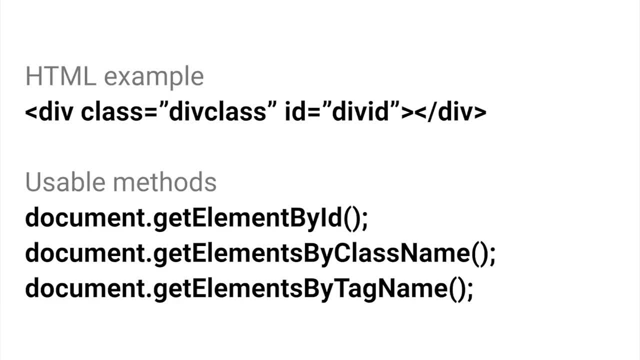 We do that by referring to the document that we have inside the browser, that is currently loaded into the browser. So by saying document dot something, we can then do something to the document. In the first example, I want to grab a certain element based off an ID. So I say: 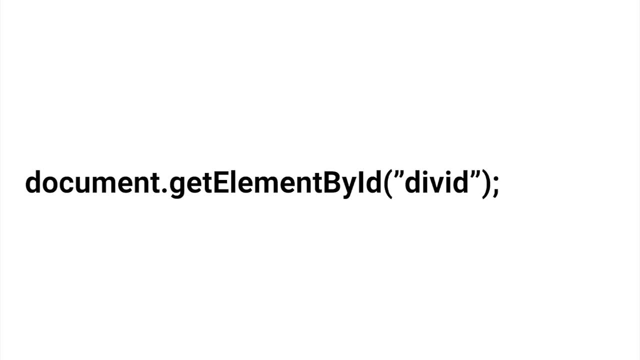 document dot get element by ID. then inside the parentheses I then refer to the ID name of the element inside the website. In the second example you can also see we can grab a element based off a class. So we can say: document dot get elements by class name Or, if you want to: 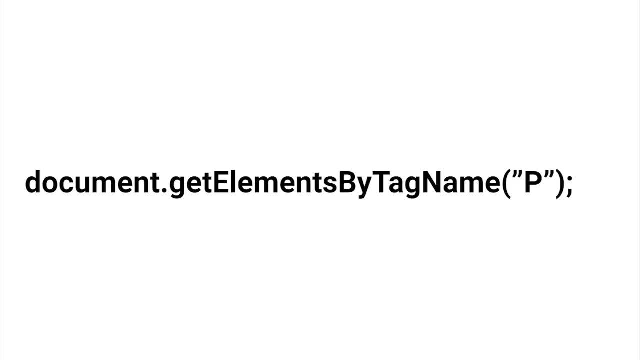 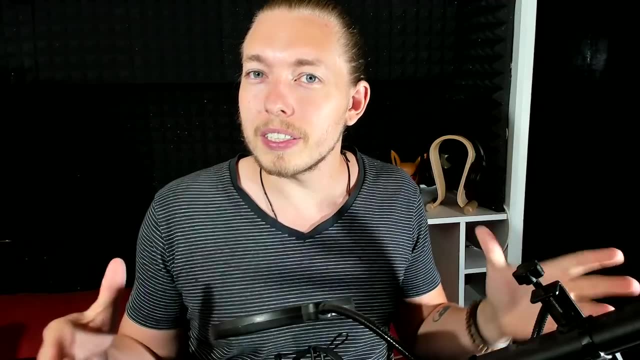 grab something by a tag name. we can also do that by saying document dot. get elements by tag name. Even though we have these methods we can use even today, we do have some new methods that are much easier to use if you want to grab something inside the DOM And you might have. 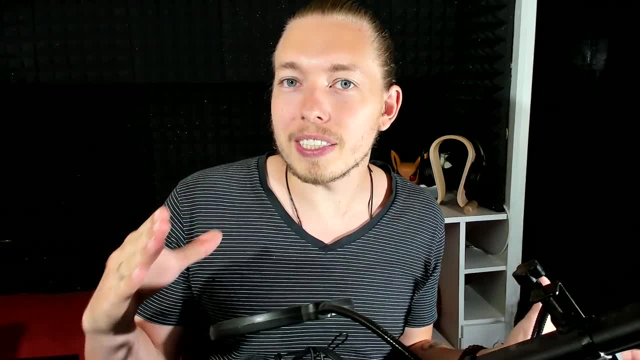 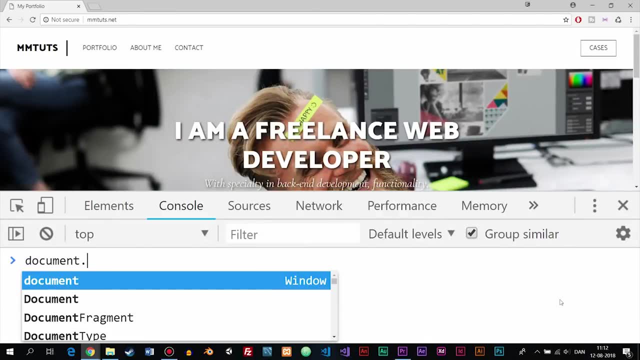 seen these methods in some of the previous episodes where we created some different projects, And these are the methods called QuerySelector and QuerySelectorAll. Now QuerySelector goes in and allow for us to grab some kind of element or a node inside the DOM by referring to either a class, 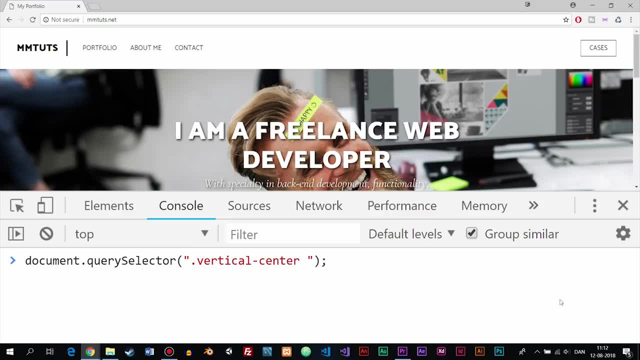 ID or tag name inside just this one method. Now the first method, called QuerySelector, allow for us to just grab one element from inside the DOM, And if we don't specify specifically which node we want to grab, it's only going to grab the first noted file. 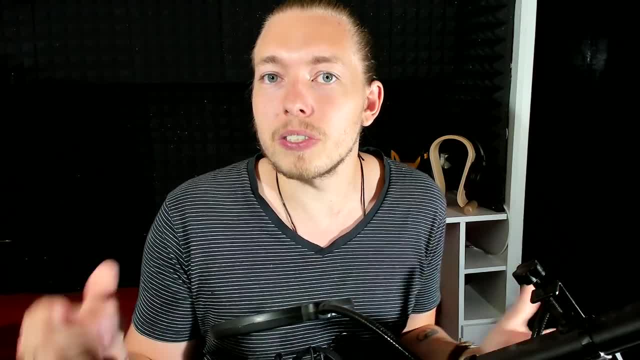 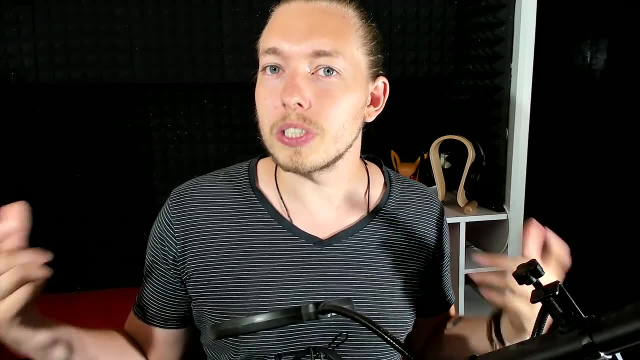 inside the DOM, Meaning that if I want to grab a anchor tag, then it's not going to grab all the anchor tags or a specific anchor tag. It is just going to grab the first one. it finds inside the website, which is the one at the top of the documents. Now, but let's say we want to grab. 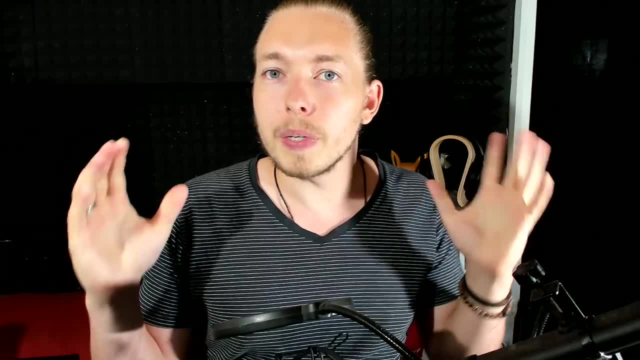 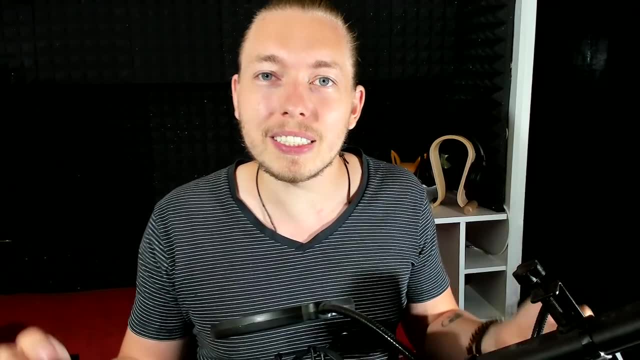 a lot of different nodes inside the DOM of the website. We can actually do that using the QuerySelectorAll method, which is going to go in and grab all the different nodes that matches the search term we put inside the method. So if I wanted to grab all the different anchor tags, 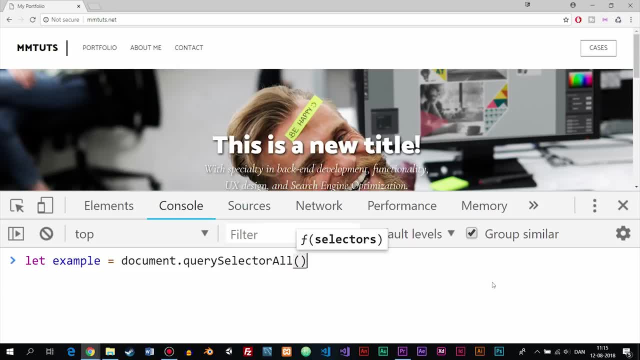 inside a website. I just need to write a inside our method And then it's going to go in and grab all the different links or anchor tags inside the website and put them inside an array so we afterwards can do something to all the different anchor tags inside the DOM. An example: